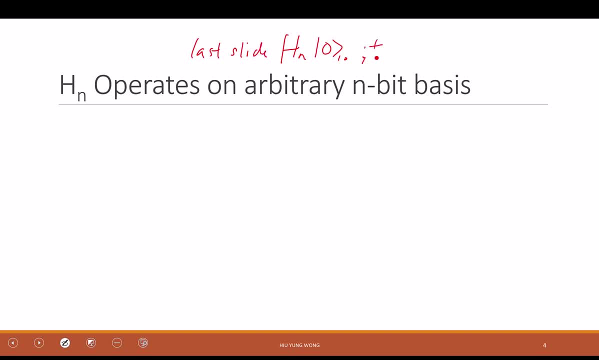 This line we're talking about applying. When I put n, it means n-dimensional Y. Do I call it Y? Yes, I call it Y. Okay. Actually, I don't want to make it confused. Yeah, let me. A 10 means decimal. 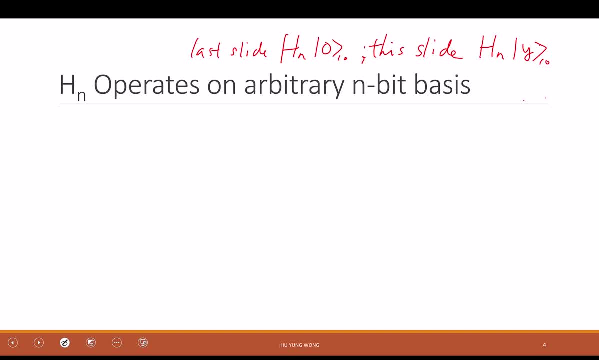 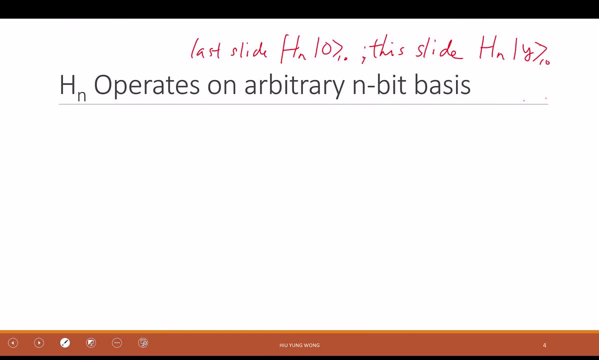 zero, The first basis vector. How about apply to other basis vector? This is what we're trying to adjust in this question, right? But in order to adjust this, it's better to understand what we mean by Y. Okay, Now Y. of course this can be in decimal. It can be, for example: 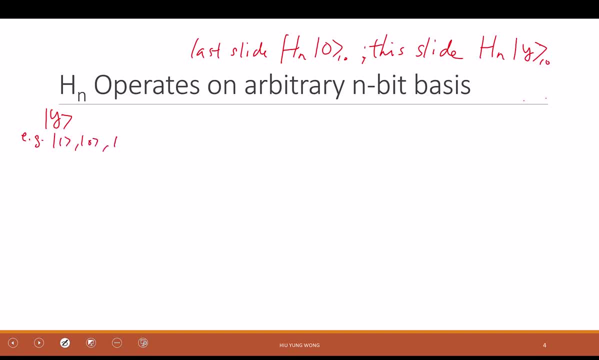 1.. It can also be 0.. It can be 9.. It can be 121 or 210.. It can be any right. This is in decimal, in decimal, But if I write it in binary I can always write it as Y n minus 1, Y n minus 2,. 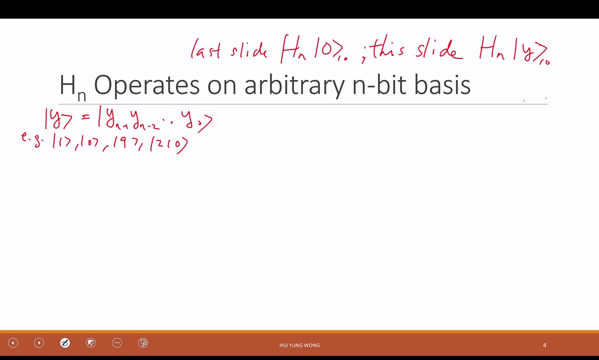 all the way to Y, zero. Okay, What does it mean? For example, it can be 1010, right. This is the case when n equal to 4.. What is this number? 0124812, right, So it is 10.. Thank you Here. Y. 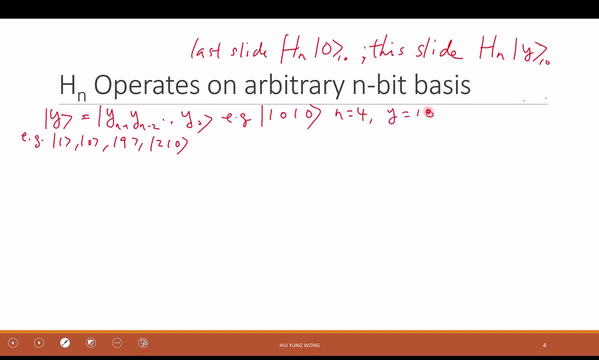 equal to 10, right, You need to have this understanding now. right, You understand. this is a label. But although it's a label, I use this. some math to help me to label it. This is the 1011 state. I come from 0.. 012345678910 of this n-qubit system. I can write it as 10 in decimal. 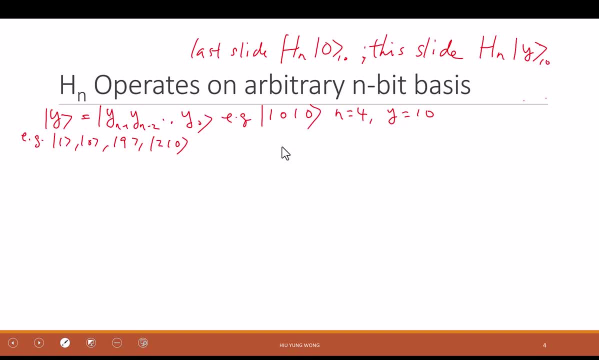 I can spell in English 10,, or I can say 11 state, or here I write 1010, because this can help me to derive the equation. Is this okay? So in summary, in decimal, what is Y right? Of course we can make it clearer Y. 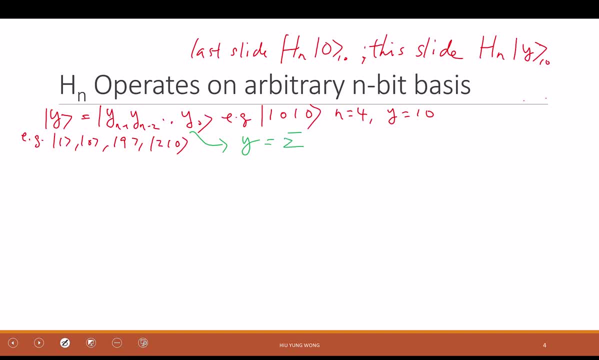 is nothing but just summation. i equal to 0 to n minus 1, Y i times 2 to the power i. I'm just repeating what I said earlier. For example, 1010 is what: 1 times 2 to the power 3 plus 0 times 2 to the power 2, plus 1 times 2 to the power 1 plus 0 times 2 to the power 0,, which is 10.. 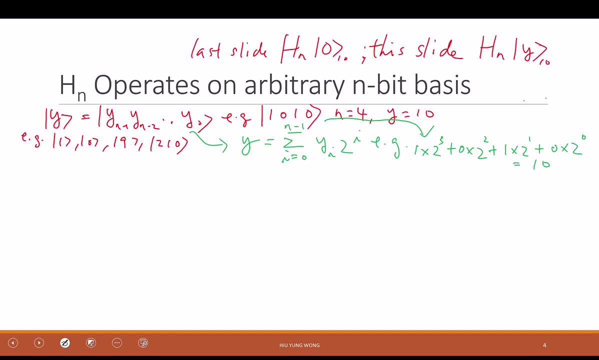 Okay, This is what we emphasize in this class: You must be able to do substitution. If you know how to do substitution, you know how to do programming. Okay, Make sense. Understand what we are talking about now. Okay, This is one of the basis state, right. 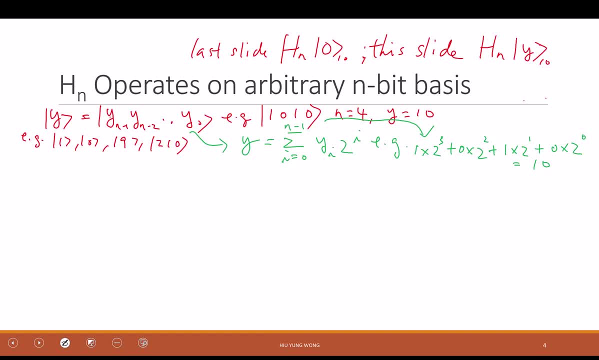 So my question is going to be super lengthy. I have two slides, so this is what we want to find out. Actually, in my cheat sheet, I also write this: I just want you to uh note that this is y3, this is y2, this is y1, this is what is this. thank you, y0. 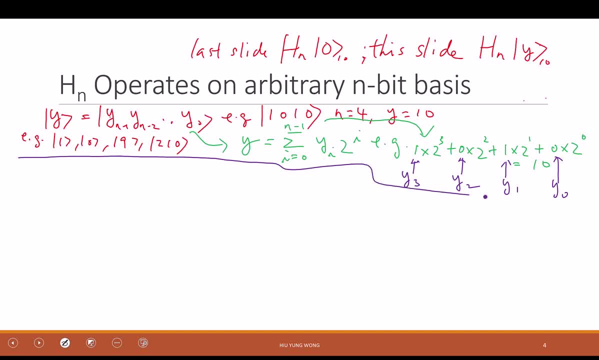 okay, but this is just a first discussion of what is y. so our goal is: what is hn operates on y, any given y. okay, then it's not difficult. now, well, we know what is y. then we say: this is just: you have h right, tensor product n time right, and then you apply the whole thing to 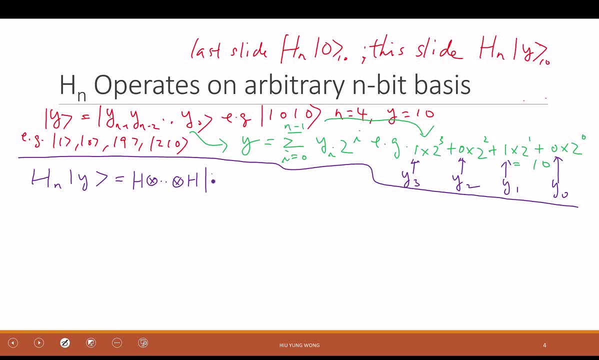 y and again, what is y? i can say it's yn minus one, yn minus two, all the way to y. zero, right, i write it in binary. and all this y, i and other, either one or zero, okay, always, if you don't know what i'm talking about, do substitution right: pick n equal to four, picking n equal to three and then substitute. 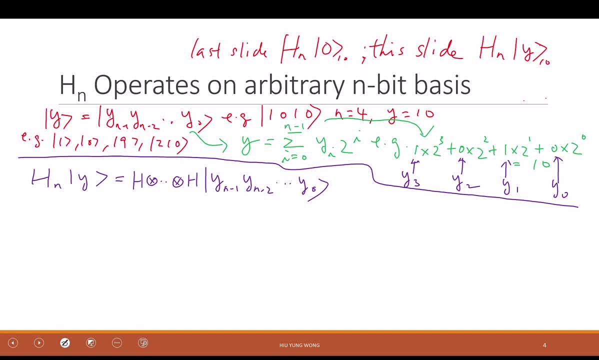 y equal to whatever number, then you know what's going on. so again, as we said, nice, this is nothing. entanglement, we can apply the hardware market to each individual subspace, right? so this is just h times y n minus one tensor product. h y n minus two tensor product, all the way to h y zero. 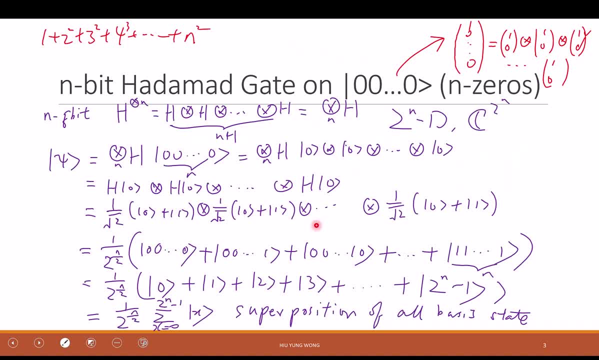 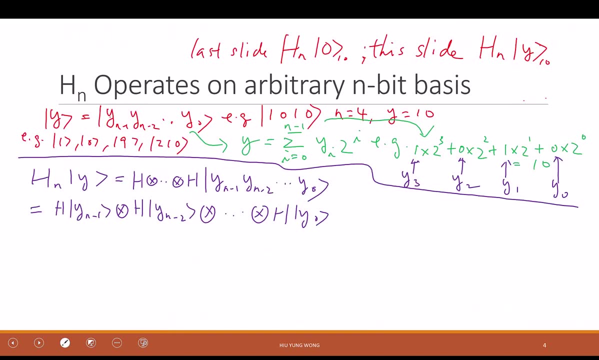 same as what we did just now for the zero case, right, except that now it's not all zero. this is a special case. y n, y, n minus one, y zero are all equal to zero, right? yeah, question? yes, because we are talking about quantum computing, i assume that all the inputs are already. 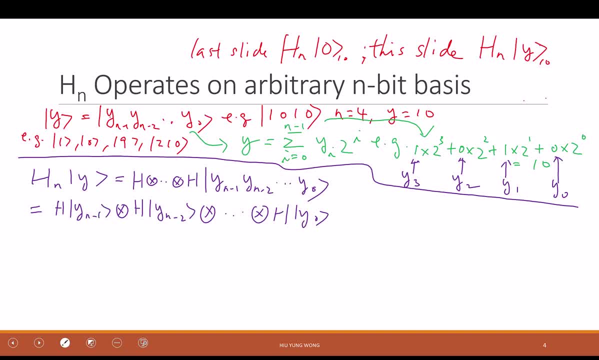 uh, normalized, right and in, indeed in all the algorithms mostly, you will start with the wet vector, zero, and that is a normalized vector. and since you are using unitary gate throughout the circuit, except you have measurement, if you have measure you're going to renormalize it. 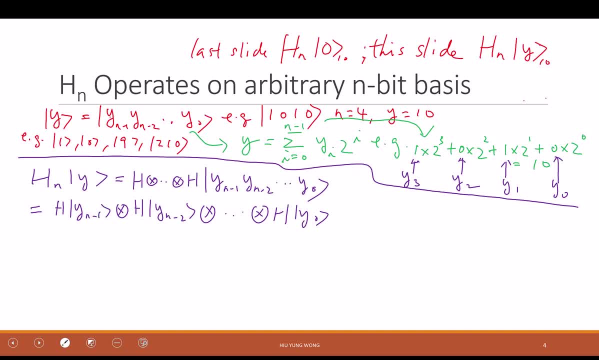 then otherwise it will be normalized all the way. yeah, so that's a great question, right? but here, when i have this basis vector, it is normalized because we only work on of a normal basis. good, good point, right? so in the exam you don't need to check. 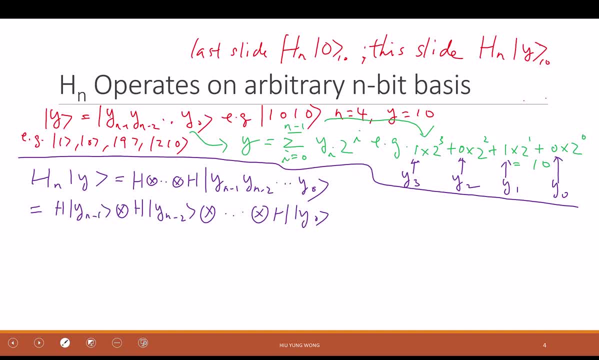 but you always ask yourself whether this is true. okay, so now what is h? h apply to y n minus 1. what then? you ask yourself: what can be y n minus 1 be? what are the possible value? 0 and and 1? you only have two value. that's why sometimes, quantum computing is. 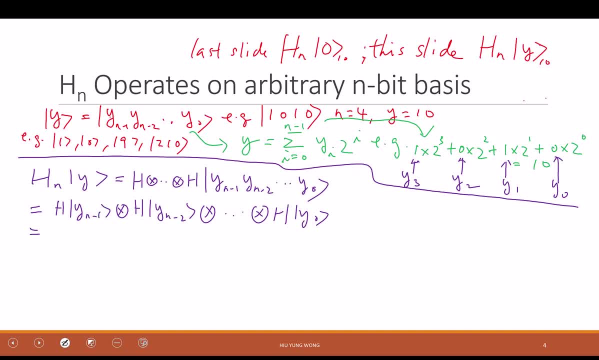 very, very easy. compared with your other classes, you only deal with 0 and 1. so if it is 0, what is the output? what is the result? h apply to 0. yeah, so let's recall: h apply to 0 is 1 over square root, 2, 0 plus 1, right, okay? what if? 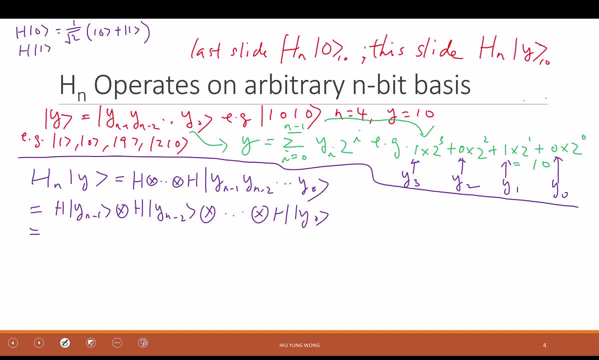 it is 1. what is that? 1 over square root. 2. state 0 minus state 1. if you forgot, fine, you have that in the chat shit, but it's time to memorize this because there are too many things. it's just like if. 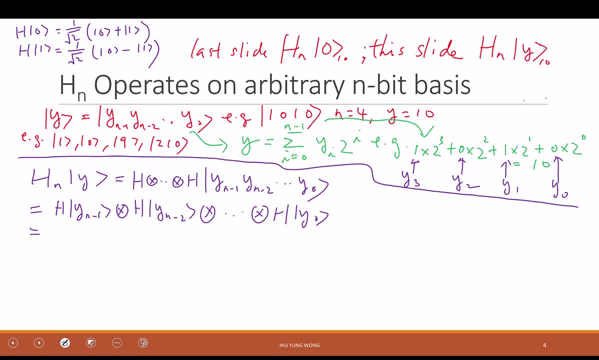 you don't know how to do multi, you cannot memorize multiplication table. it make your life more difficult, although nowadays the educators say, ah, don't memorize too much. it's just that if they want, you keep memorizing and forgot the goal of learning. but if you 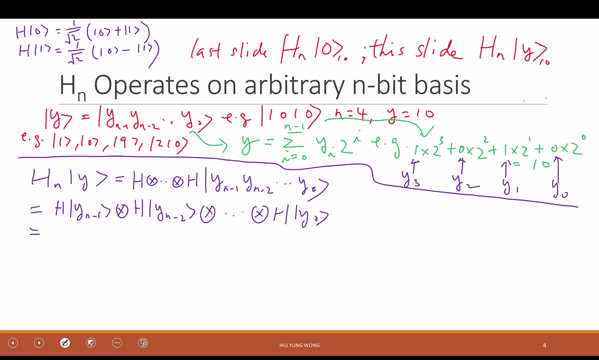 don't lose the goal. it's better to memorize, right? so now it's time to memorize. how can i make this as an equation? right, because i don't know whether it's zero or one. right, because why? n minus 1 can be 0 or 1. any suggestion? what is h applied to y-1? how would you let's? 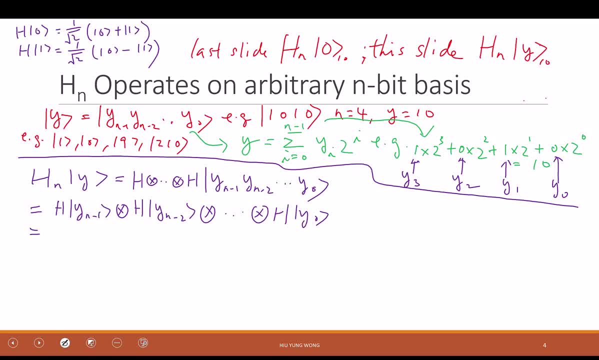 say you need to write a program, how are you going to program it? very good, let me. let me slow you down. coefficients are the same, so we can write it as it is. and then, what change is the size? so i basically also can write it how: what is your self- costumes? 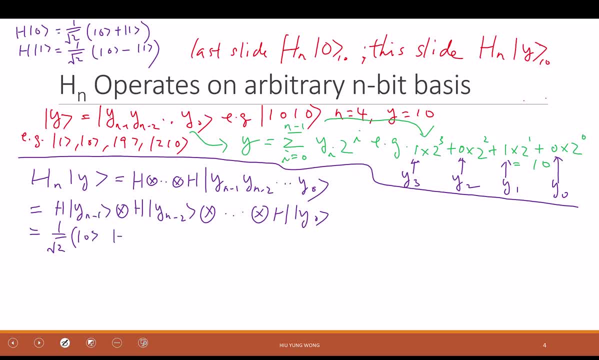 �에 this. it's just that I need to think about how to deal with the sign. but if you are writing a program- or actually you already know mathematically- how can I write something so that it is correct but depends on y, n minus 1, huh. 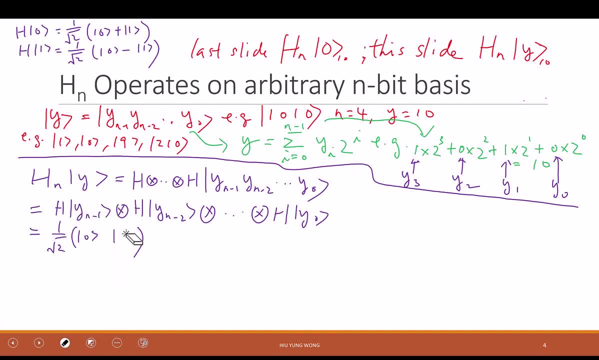 exponent right, so you can do. let me write this wider. yeah, so this one. you just need to learn it one time, then you can. you know how to use it forever, do you agree? it's negative 1 to the power y n minus 1. if y n minus 1 is 0, you get 1. 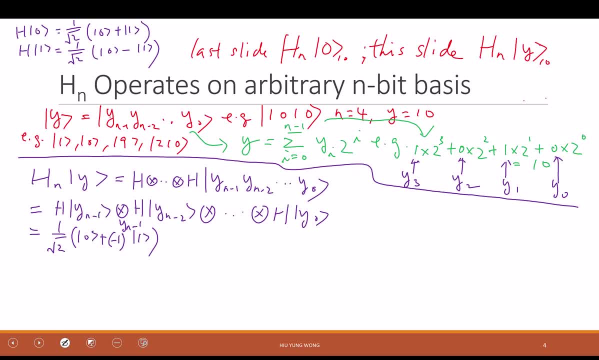 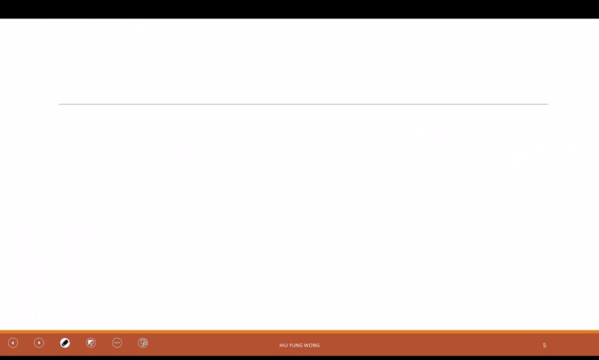 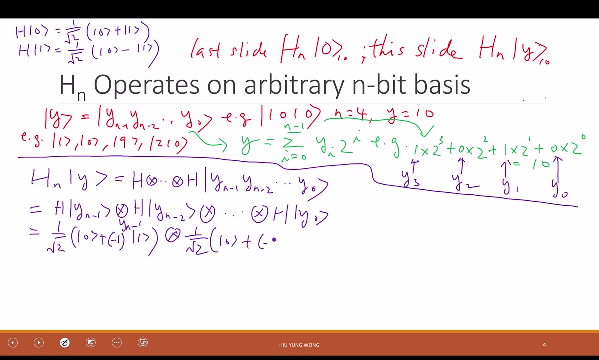 right. if it is 1, you get negative 1 right, then I'm success. I successfully written the equation. it's general right. so the same thing happened to others. is equal to 1 over square root, 2, 0 plus negative 1, y n minus 2, and then 1, and I continue, I keep going, and then I. 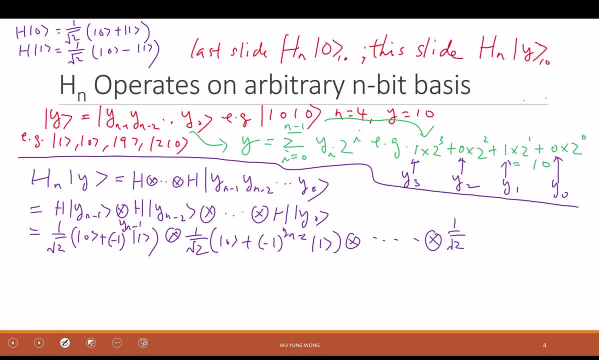 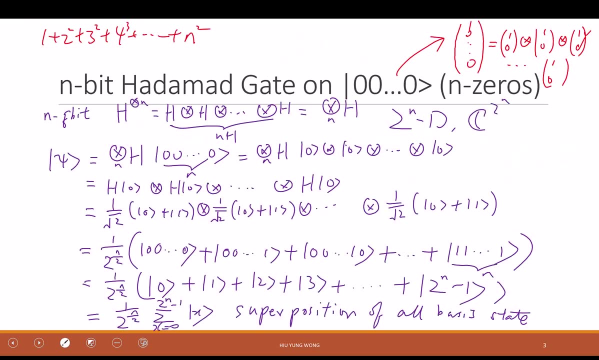 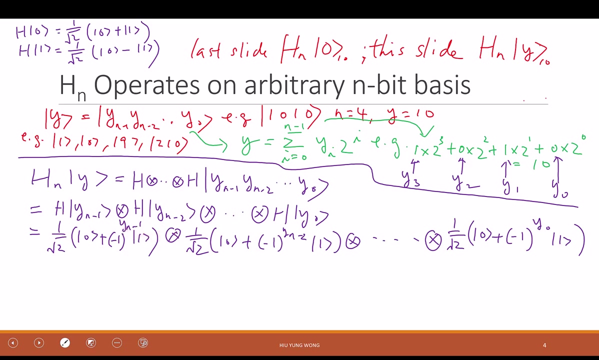 say the last one is 1 over square root 2. 0 plus negative 1. y 0, 1 x, 1 over square root 2 is exactly what we did for the zero basis. look at this: this is exactly the same, except that this time it is not all 0, the y1 yi can. 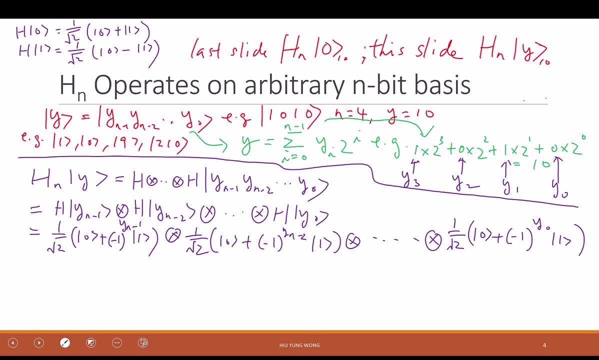 be 1. when this is 1, we need to put negative. then what is the next step? just express it right. first of all, just like the zero basis, it is exactly what we did. case this is equal to 2 to the power n divided by 2, because I do have 2 to the power n terms. 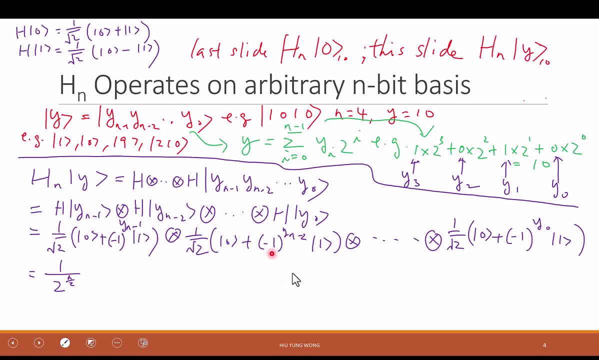 when I multiply, not 2, to the power n terms, I have n terms right 1, n. 1 over square root 2, so I have 1 over 2, n divided by 2 because of square root 2, okay, Then I'm going to multiply. 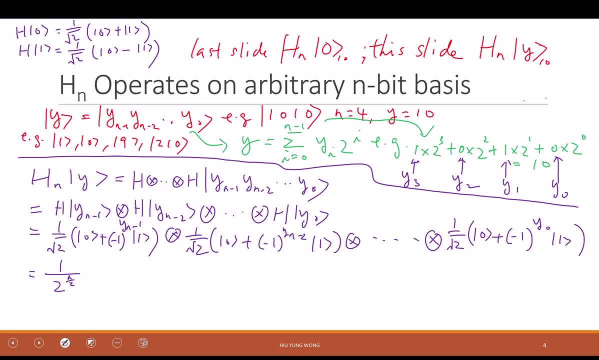 them. It's not too difficult This one at this stage. do not difficult. I start with 0.. What are the coefficients for 0?? What are the coefficients for 0?? It is all 0, right. I mean all 1, right. 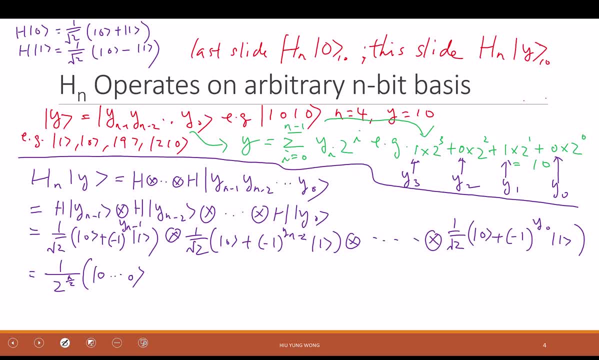 Make sense Now, but I deliberately going to do this. When it is 0, I just multiply them. I try to put negative 1 to the power 0 to it to help me to understand better later. This is just 1.. So whenever I have a 0,, I put negative 1 to the power 0,, which is 1, right. 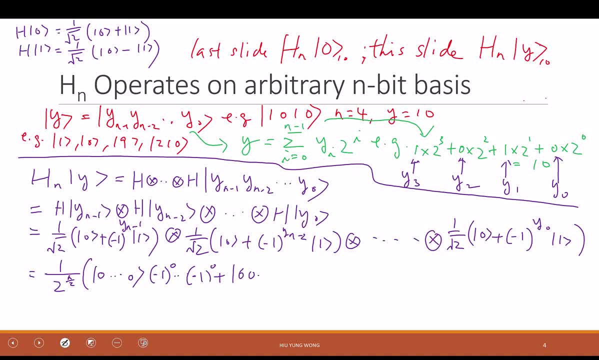 How about the second term? I still have 0, 0 all the way to 1.. Again, for every 0, I put a negative 1, but when I see the 1,, I need to put negative 1 to the power y 0. Do you agree? Because this times, this times, 0,. 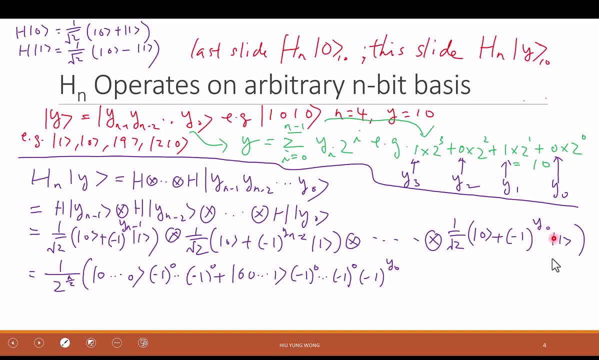 and then the other. the last one is 1,. right, So I have negative power, negative 1 to the power y 0.. Make sense? What I'm trying to show you is that I hope you to recognize that whenever you have 0,. 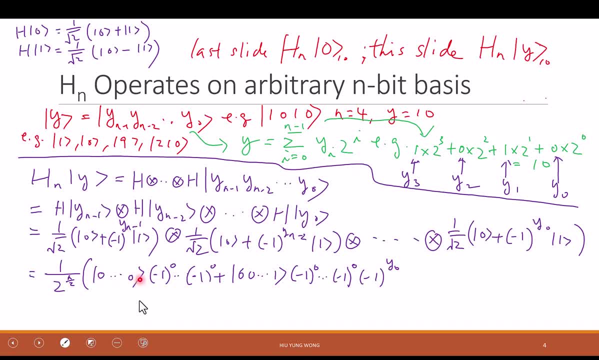 it's negative 1 to the power 0 associated with this term, And if you have a 1 inside, it's negative 1 to the power y and depends on the location of the 1.. Ah, then you know whether it's negative 1 to the power y 0 or y 1 or whatever. 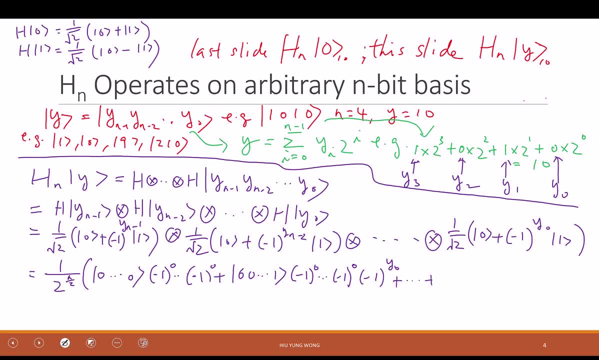 What is the last term? What is the last term when you expand this? What's the last term? 1.. 1,, 1,, all the way to 1? Then what are the coefficients? 1, 1,, all the way to 1? Then what are the coefficients? 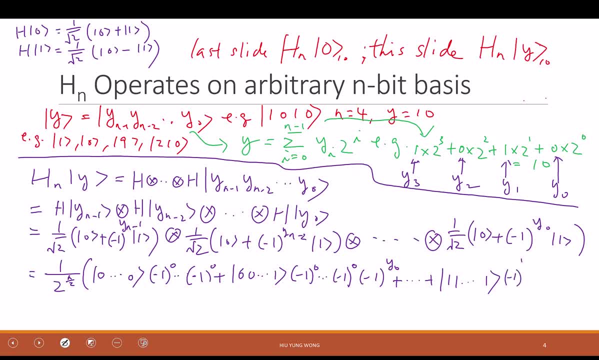 Negative 1, y n minus 1, negative 1, y n minus 2,, all the way to negative 1, y 0, right, Is this okay? I add this is to make it easier later. 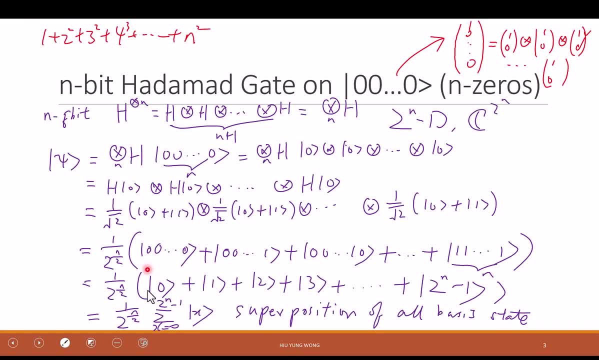 The point is the same like what we did for the 0 case. For the 0 case, we also say: you just multiply and then you get this: 0, 0,, 0,, 0, 1, all the way to 1, 1,, 1,, 1, 1, right. 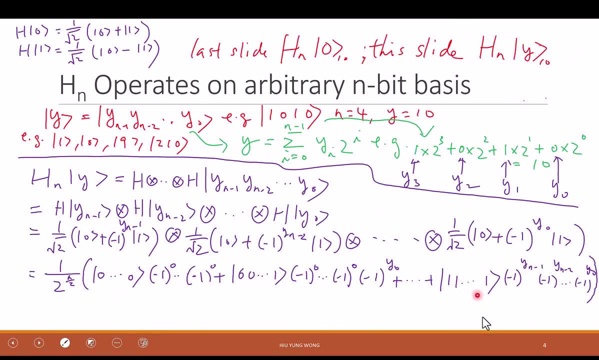 This is same here. I get 0,, 0,, 1, and then all the way to 1, 1,, 1,, 1,, 1, 1.. But I still have this coefficient to deal with For 0,. I always put 1,, which is negative 1, to the power 0. 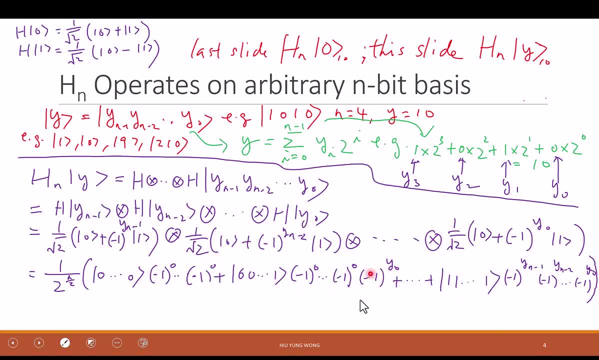 I deliberately do that. And then for 1, it will be negative 1 to the power, y, 0.. It depends on where you put the i. right, Is this okay? Now let me write this one more time, Or maybe I don't write this right. 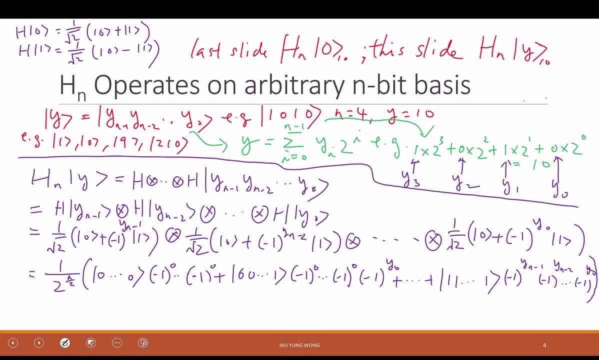 If now, now, our goal is to determine what are these values? Now, I call: this is 1,. no problem, This is 0,. right, This is 1.. And what is the value of the last term? 0 to the power n minus 1.. 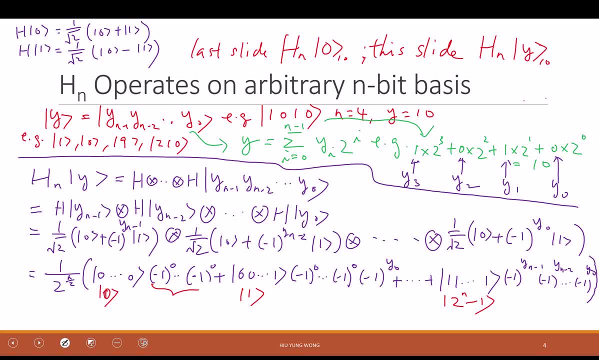 I can write them as that, But my goal is that. so, again, it's a superposition of all the terms. Do you see that? The only difference is that I don't know the coefficient. What are these? Okay, If I call this, I call this C0, C1,, C2.. 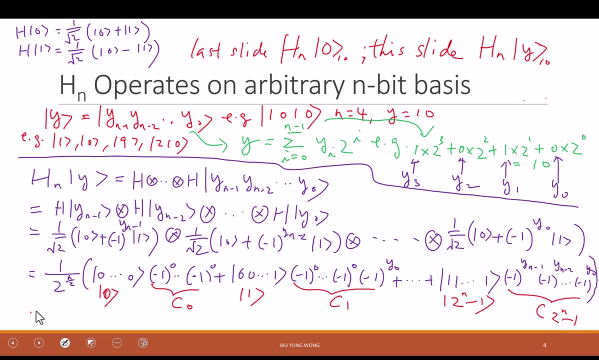 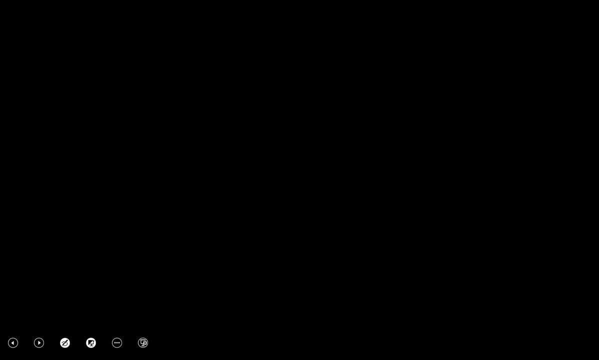 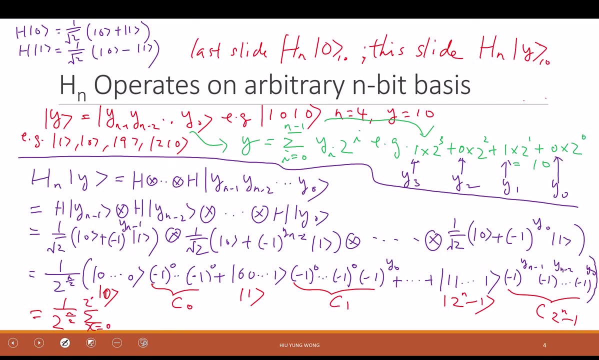 2 to the power n minus 1.. Isn't that this is just 1 over 2 to the power n over 2?? Summation: x equal to 0 to the power n minus 1, x times Cx. Do you agree with what I'm saying? 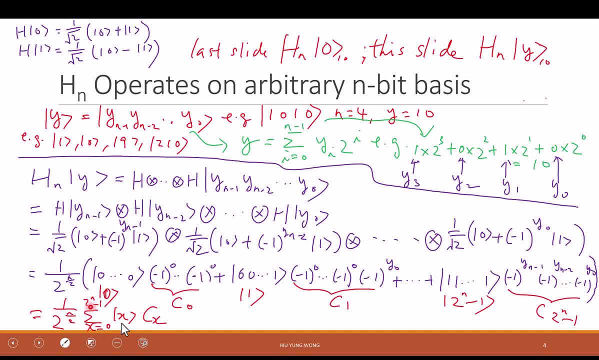 I am not. I am not calculating the coefficient yet, I just write the sum. I call the coefficient C0, C1 to C2, to the power, 2 n minus 1.. This is just the sum of all the x, all the superposition right. 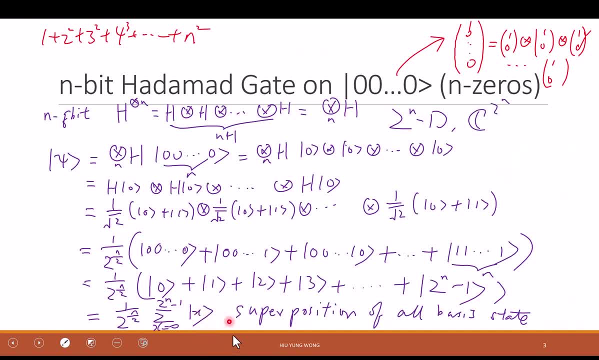 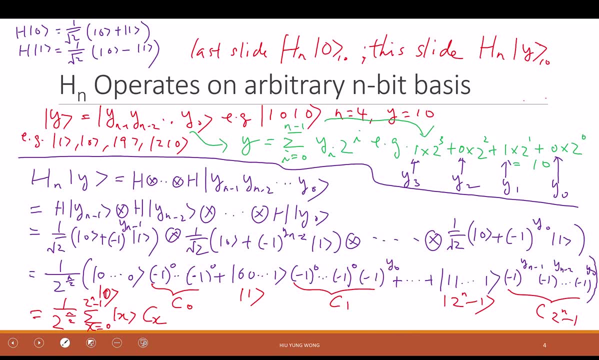 It's the same form, Exactly the same Superposition of x, Because all the math are the same. the only problematic thing is I need to find out what are the coefficient. Okay, Everything is the same. So it's still a superposition, but it might not be equal. 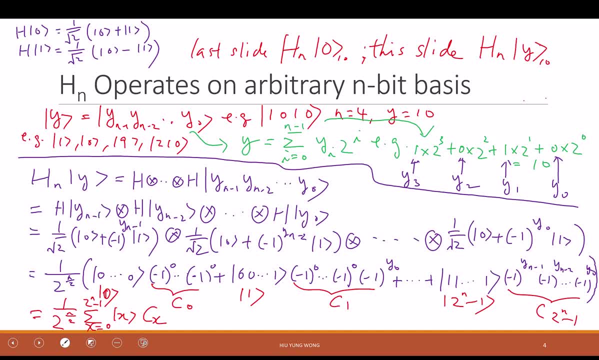 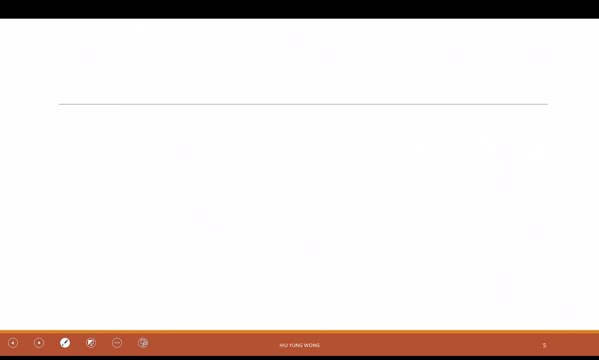 In terms of magnitude it's equal, however, But their phase are not the same. Okay, So our goal, the next step is to understand what are the possible, what are the value right. So what are C0, C1, all the way to power, C2, to the power n minus 1.. 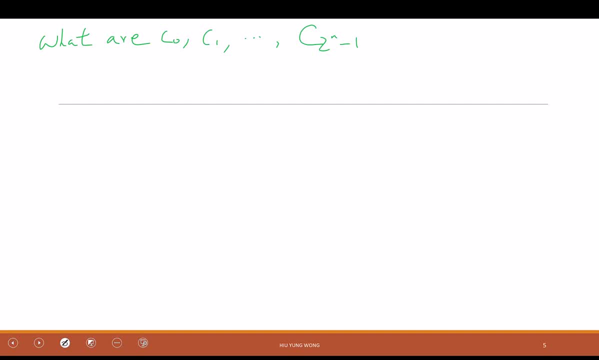 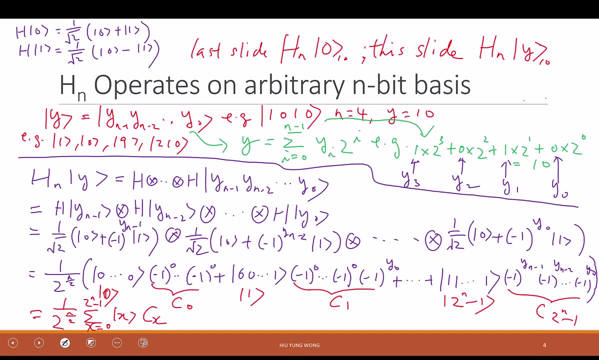 Okay, Now you find that this is a little bit Confusing, Right? How do you get it can be. if you look at this, what are the possible value? What can be the possible value if you have negative 1 times something? 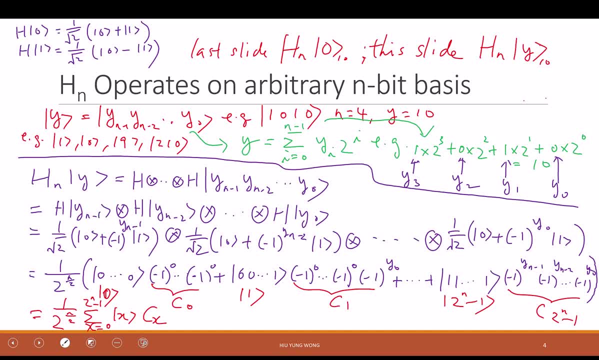 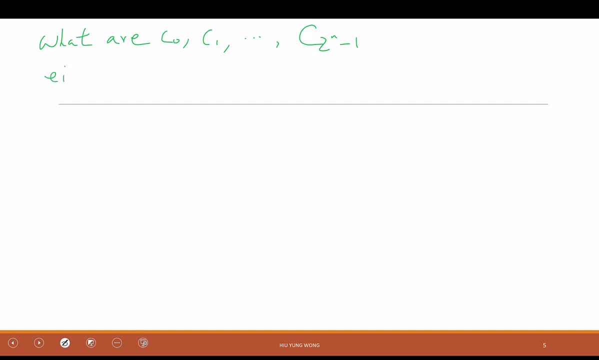 Negative 1 to the power something times negative 1 to the power something. What are the possible value? Yes, either plus 1 or a negative 1, right, Just because of the math, Right, But where you will get negative 1, right. 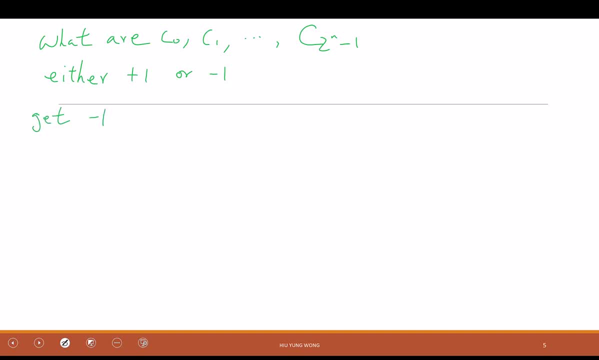 You will get- let me write down- negative 1 if xj equal to 1 and yj equal to 1.. Okay, This is the first term, Not the whole thing. negative 1, right, You will get negative 1 for one term. 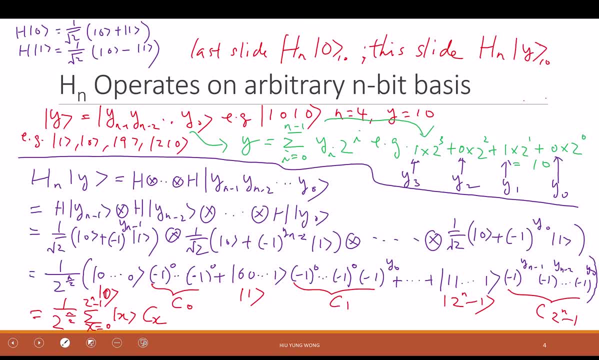 What do I mean? First of all, you want to get negative 1.. You, this is the xj, Right, This is the x. So each of them. if your x is 0, then the coefficient is negative: 1 to the power: 0. 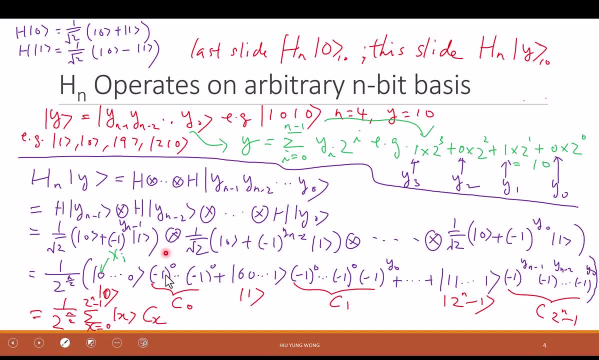 You are not getting negative 1 because it's contributing Right. You only will get a negative 1 from there if you actually have a 1 in the xj, Because you then have a coefficient which is negative 1 to the power i- yj. 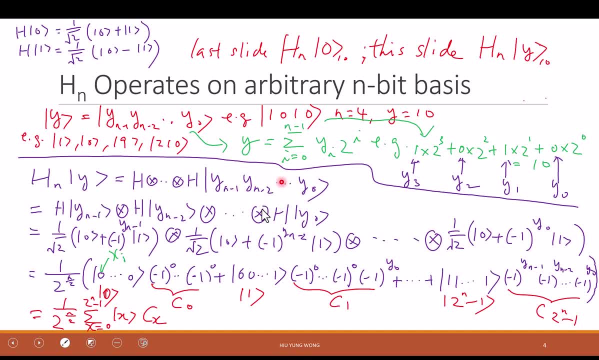 But if your yj is 0, because y can be 0,, it doesn't have to be 1.. Okay, Then you still get 1,, not negative 1.. So you, for each of this term you need to have right. 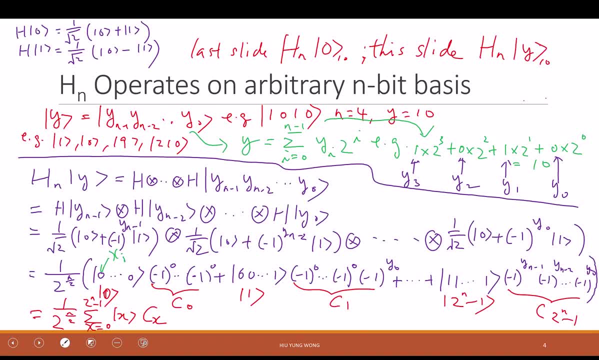 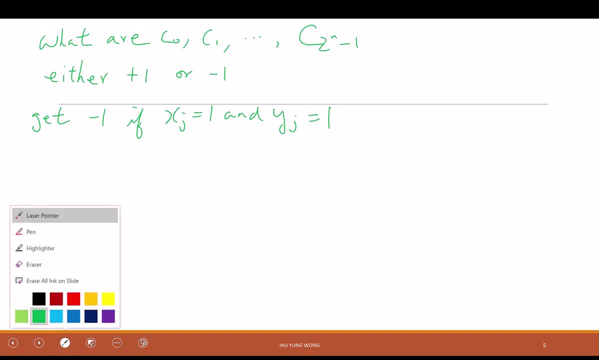 So I need to make it clearer How to say: Yeah, You. let me rewrite this sentence. I should say: You get. You get a contribution of negative 1 to the coefficient. It's just a contribution If xj equal to 1 and yj equal to 1.. 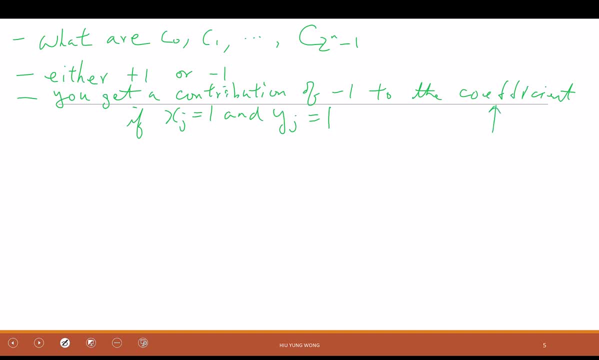 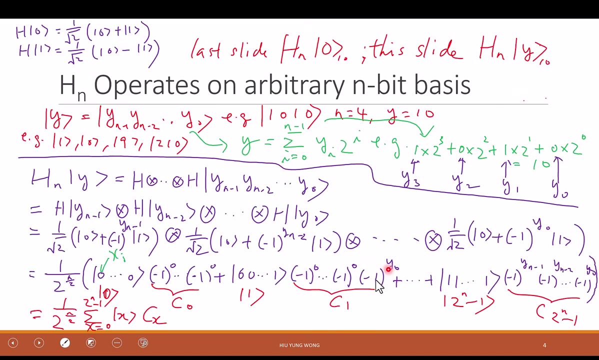 Okay. What do I mean by coefficient? This is the coefficient C 0. C i, Let me call it C i. Okay, Okay, Coefficient, For example, we are looking at this one. You want to get a contribution of negative 1.. 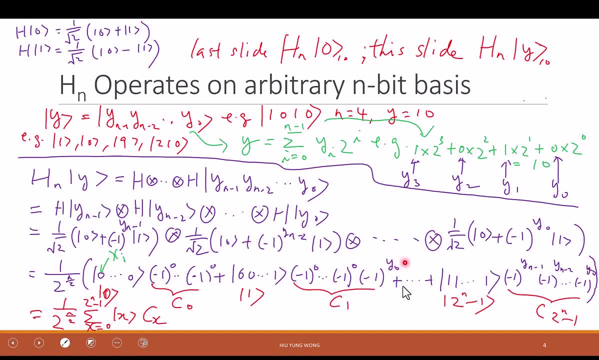 You need to have x1, xj equal to 1, and yj equal to 1.. Right This x0 equal to 1, and then y0 also 1.. Then you get a negative 1. Because if your x0 is 0,, I have negative 1 to the power 0. 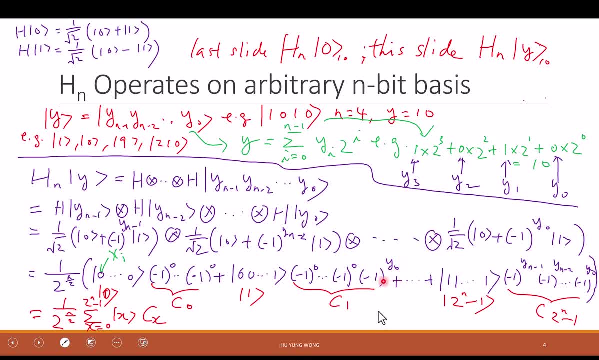 And if your y0 is 0, I have negative 1 to the power 0. And if my y0 is 0, this one is also give me 1.. So I don't have contribution. So how can I get a negative 1 for the whole coefficient? 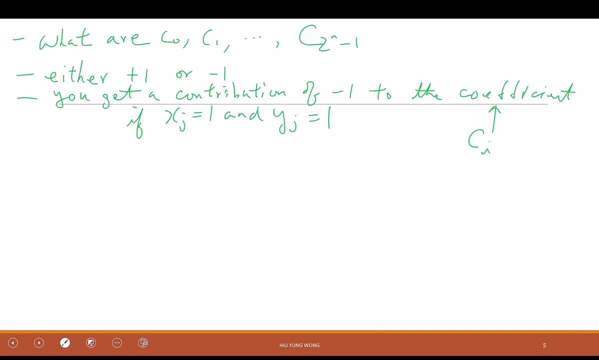 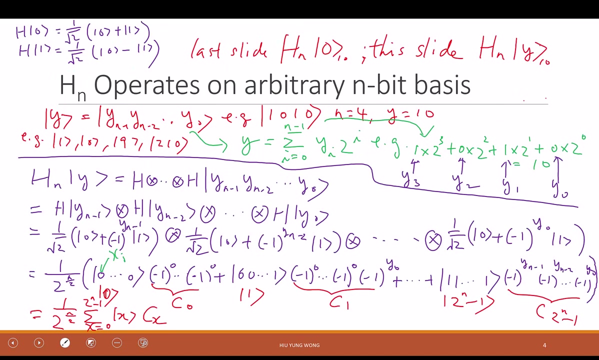 I need odd number of this term, Okay, Okay, And then need odd number of such contribution. Sorry for my writing. To get C i equal to negative 1.. Right, Because if I only have two terms, that is negative 1, they will become 1 after multiplication. 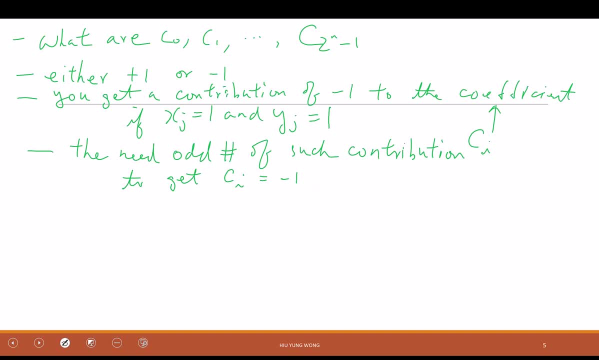 Right, So how do we write this? Then? it means basically: you want to do C? i Is equal to Negative, 1 to the power. x dot y. Okay, Okay, It's the meaning: of x dot y. Let me show you. 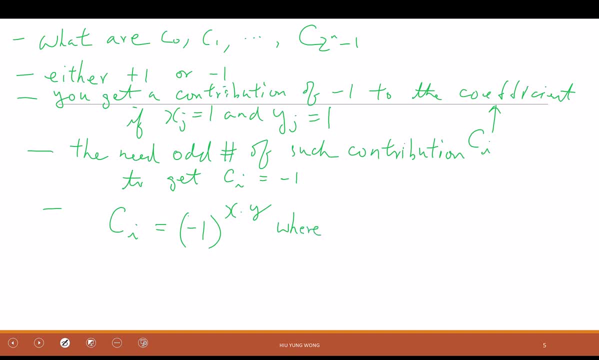 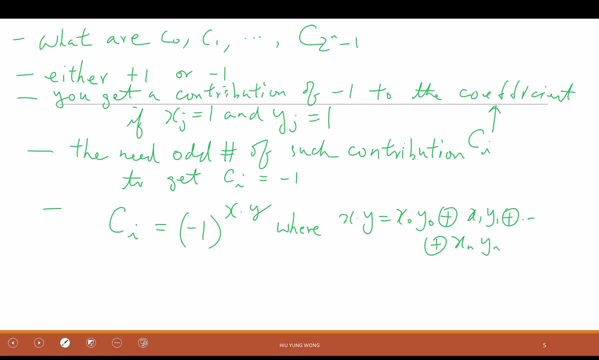 Basically here you think that because if x times y, we say need to both as 1, right, Then you are going to have 1.. And exclusive is counting how many 1.. Exclusive binary string is counting how many 1.. 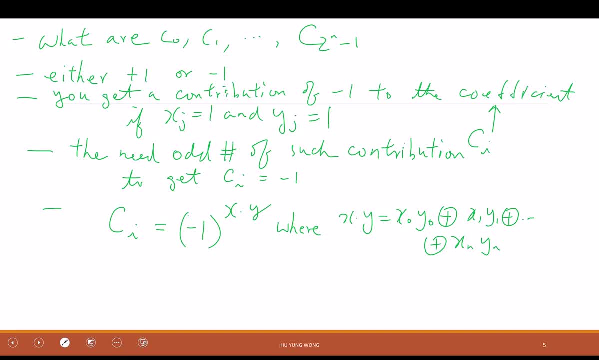 Right, Right, If you have 1.. Whether it is odd or even number of 1.. If it is odd number of 1, you get 0.. Excuse me, you get 1.. If it is even number of 1, you get 0.. 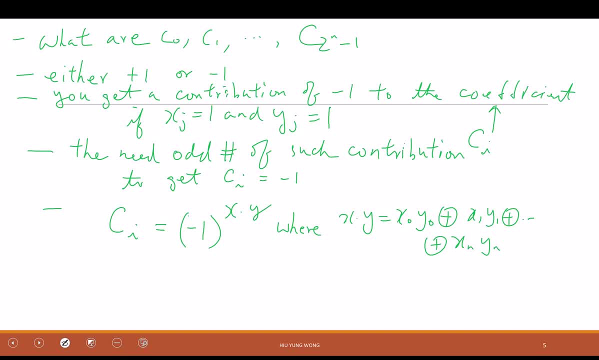 So this 1, it's just counting odd or even number of xi. Like I call xj, y, j equals to. like I call xj y, j equals to. like i call xj y, j equals to. 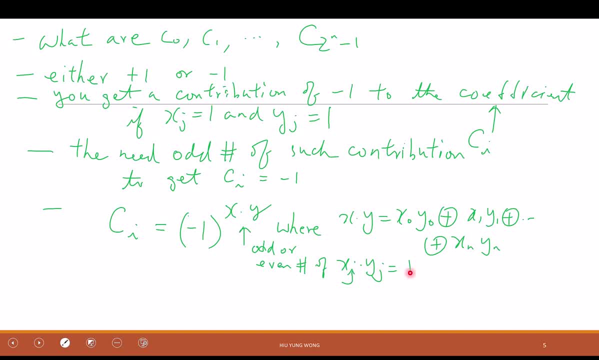 1, because each of this pair gives me a negative 1. okay, then, in summary, I have this: when I apply the Hadamard gate to an n-cubit, y, n-cubit is equal to 1 over 2, to the power n over 2. 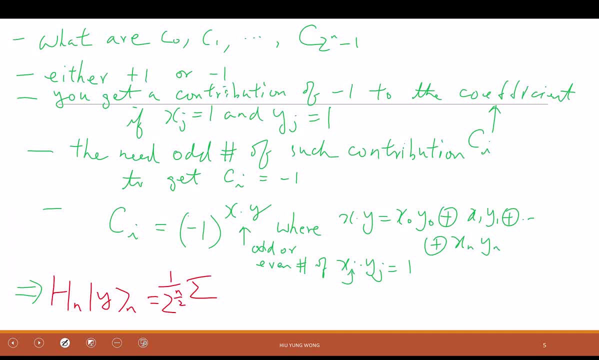 x equal to 0, 2 to the power n minus 2 x superposition of all the basis states. but the coefficient is negative. 1 x dot y, which is just like an inner product. okay, but let's do not talk about inner product. if you think about modulus, then it is just inner product. 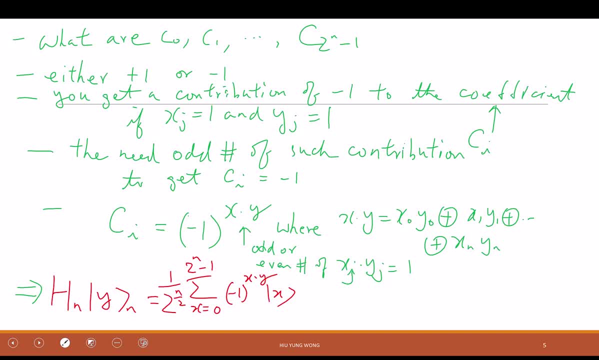 but just think about that, the bitwise of the n-cubit y- n-cubit y operation. okay, any questions now I don't think that you will understand right away. looks like every step is okay. right, the best thing is to do substitution. okay, that's what I'm going to do. but here just remind you that. 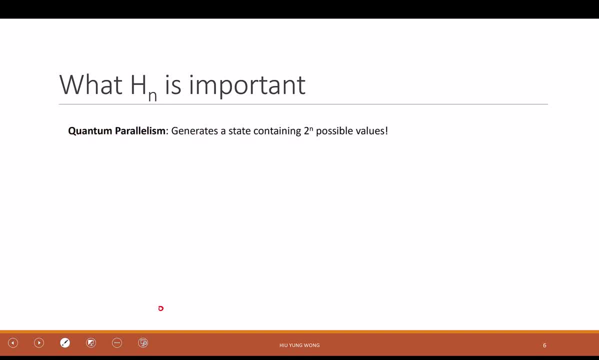 quantum parallelism is enabled by the Hadamard gate. you can do the superposition. let's try to calculate the h of the n-cubit y operation. right, the first one. the first method is this: I want to apply h2, which two qubit, to one one. okay, so this one. I'm using this method. 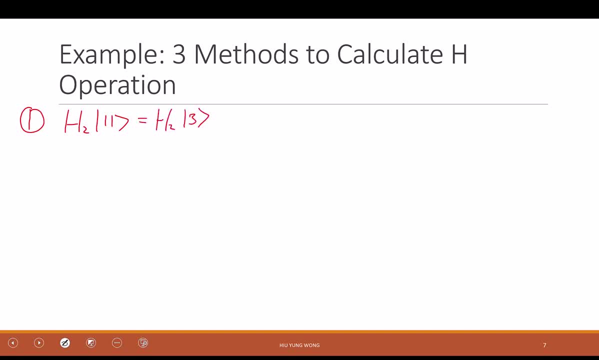 this is called h2 applied to three right, I just let you know this is three. so if I look at what I just said, right we have. this is just nine h n applied to y, with n equal to what and y equal to what, n equal to two to two qubit and y equal to. 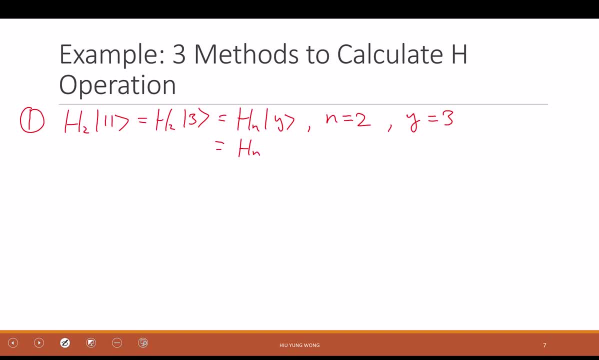 three right, which is equal to- I know I'm repeating- y1- y0. what is y1 one? what's y zero one, right? I want you to be able to recognize this. okay, now, this is actually. this is not the method, yet this is the goal, sorry, okay. so let's start with one. 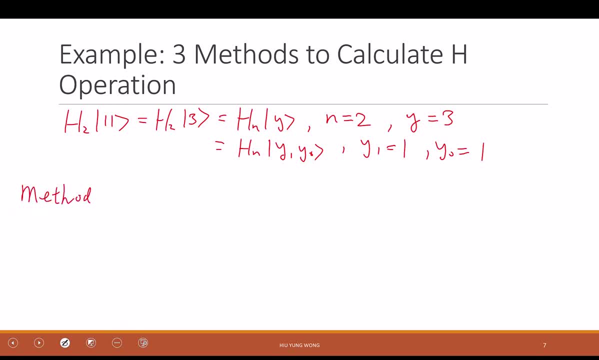 method. method one, we use the simple one. we start with H, 2, 1, 1. we say let me do it individually in the subspace. let's say I have not learned the equation make sense. I break the two qubit. Hadamard gate. apply individual to subspace right. 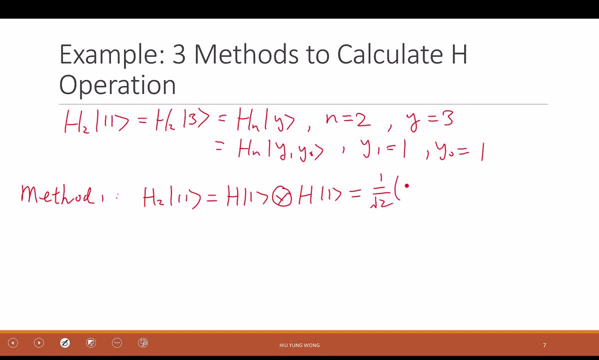 so what is this? 1 over square root, 2, 0 minus 1. tensor product: 1 over square root 2, 0 minus 1 equals to what? 1 over 2? right, just do the multiplication 00 minus 01 minus 10 plus 1: 1. 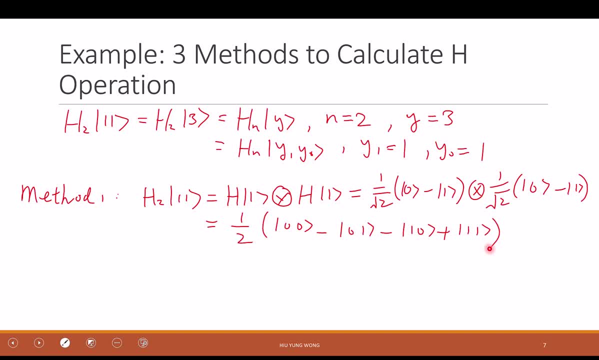 everyone follow nothing right: 0, 0 negative. 1 times 1 negative. 1 times 0, 0 times negative. 1 negative 1 times 0, 0 before. and then second addition equals. next addition equals 0, another one now we will find here: equals 1 minus 2 minus 2. 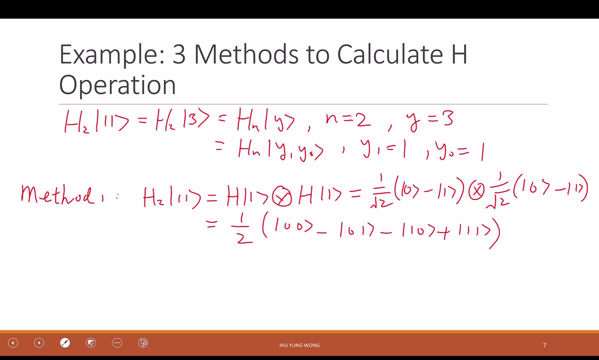 negative one, so that's why you have plus here and minus here. okay, so this is first method. you know how to do it already, right before this class. if I already told you this definition, right, you know very well. method two: what we can do is: how many method do I have actually? okay, I am going to use the 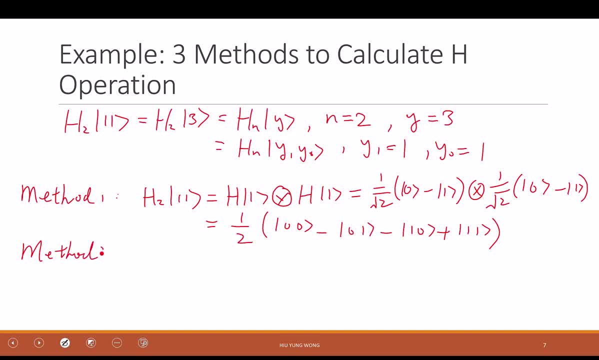 equation. yes, you can. yeah, but now I'm going to use the equation we just learned. okay, h2 applied to 3 equals to summation x, equal to 0 to 2 to the power n minus 1. I have no space, I just put here 2 to the power n divided by 2. 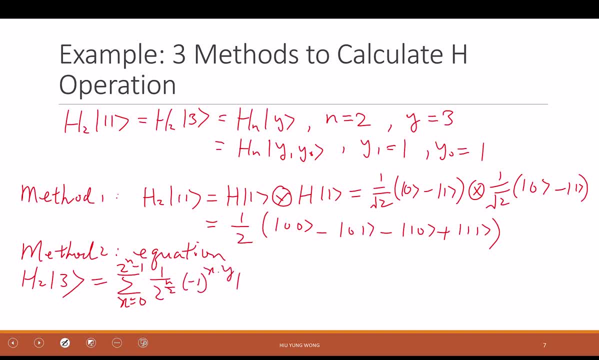 and I have no space, I just put here 2 to the power n divided by 2, and I have no space, I just put here 2 to the power n divided by 2 and negative 1 x dot y x. this was the equation I just 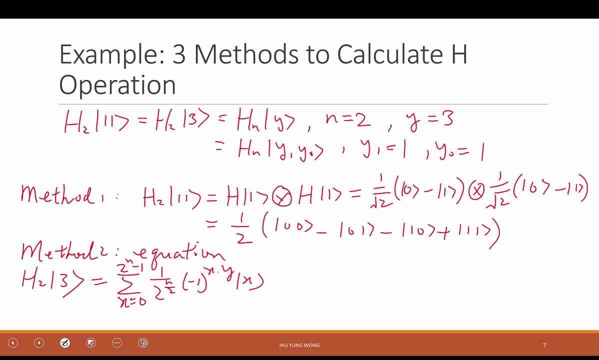 negative: 1 x- dot y x. this was the equation. I just negative: 1 x, dot y x. this was the equation I just show you. is this okay? but what is show you? is this okay? but what is show you? is this okay? but what is n? and it's 2 right. so this is 1 over 2, 1 over. n and it's 2 right, so this is 1 over 2. 1 over n and it's 2 right, so this is 1 over 2. 1 over 2 to the power. n over 2 is 1 over 2. 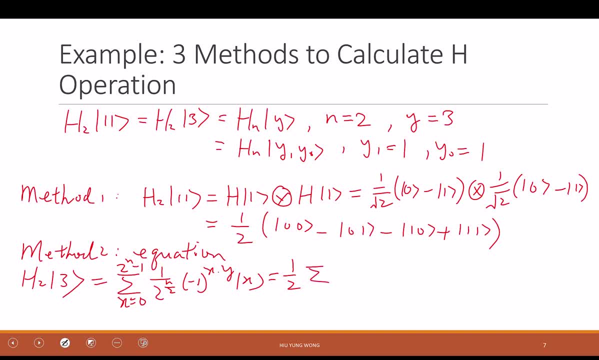 2 to the power n over 2 is 1 over 2 because n is 2 and summation is what to? because n is 2, and summation is what to? because n is 2 and summation is what to the power 2 minus 1. so this is 3, this is: 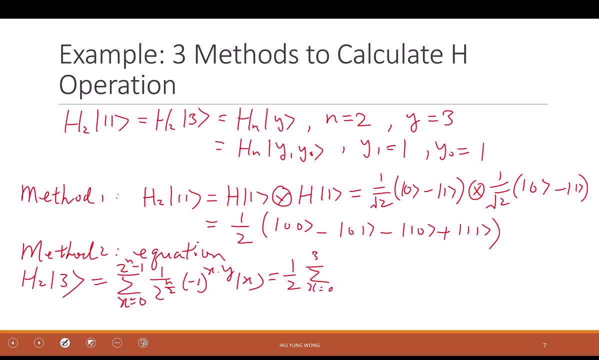 the power 2 minus 1, so this is 3. this is the power 2 minus 1, so this is 3. this is what you need to do in the homework, what you need to do in the homework, what you need to do in the homework that I asked you to do in question 10 and. 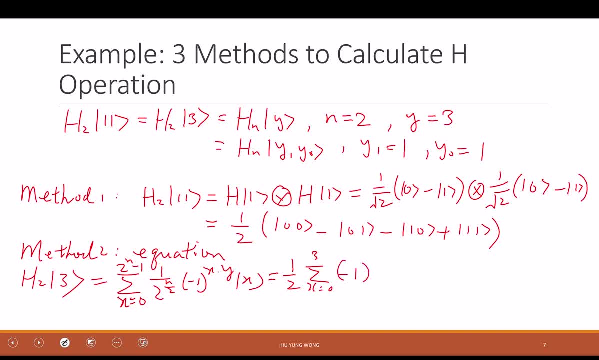 that I asked you to do in question 10 and that I asked you to do in question 10, and then I have negative 1. what is y 3, 3? then I have negative 1. what is y 3, 3? then I have negative 1. what is y 3, 3, dot X. okay, I can expand it, so it is. 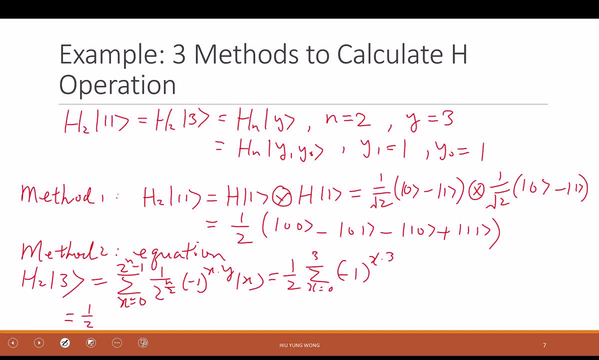 dot X. okay, I can expand it. so it is dot X. okay, I can expand it, so it is clearer. I start with X 0 0 is basically clearer. I start with X 0 0 is basically clearer. I start with X 0 0 is basically: is 1 over 2 times X. I am missing this. 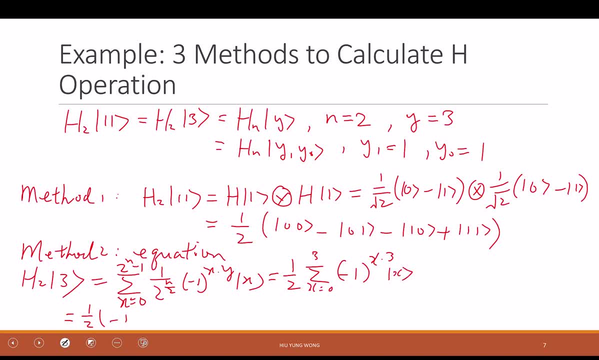 is 1 over 2 times X. I am missing this is 1 over 2 times X. I am missing this one right X: negative: 1 0 0.3 0 plus. negative: 1 1.3 0 plus 0.3 0 plus negative: 1 1.3 0 plus. 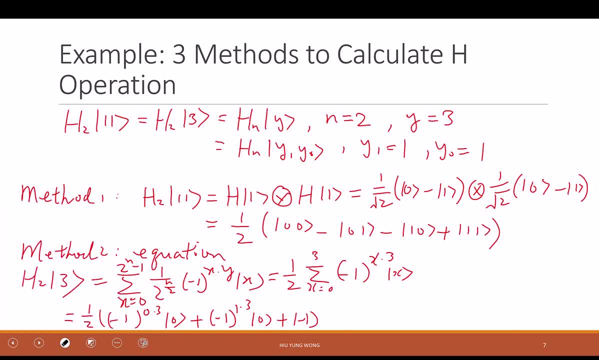 0.3 0 plus negative. 1 1.3 0 plus negative. 1 huh negative. yes, this is 1 thank you, that is negative. yes, this is 1 thank you, that is negative. yes, this is 1 thank you, that is 1. X is 1, 2.3 2 plus negative. 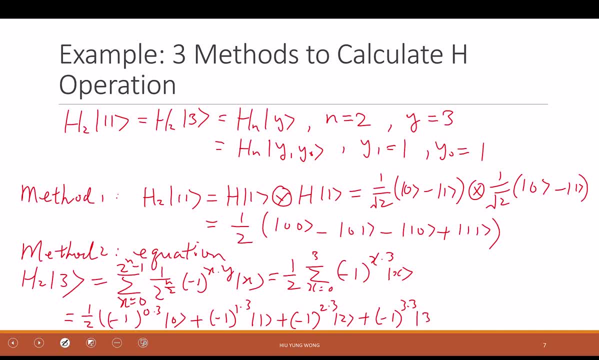 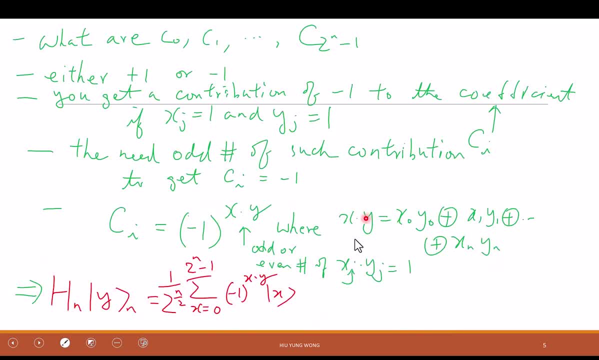 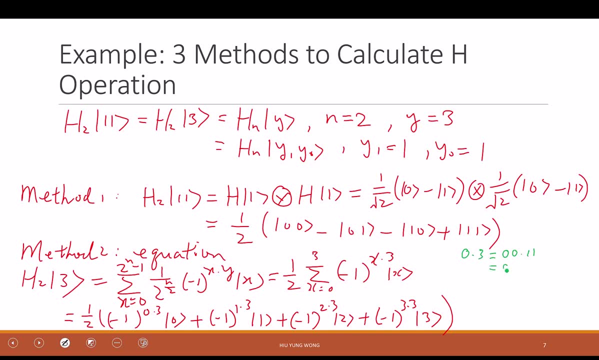 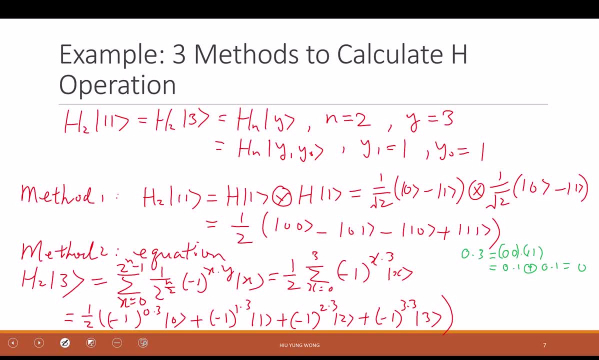 one. this is even zero, one right. what is one dot three, then? well, one is zero one, three is one one. so, using that equation: is zero dot one, exclusive one dot one. what is this? it's one right. you only have one, because the first term is zero, right. two dot three is one zero. 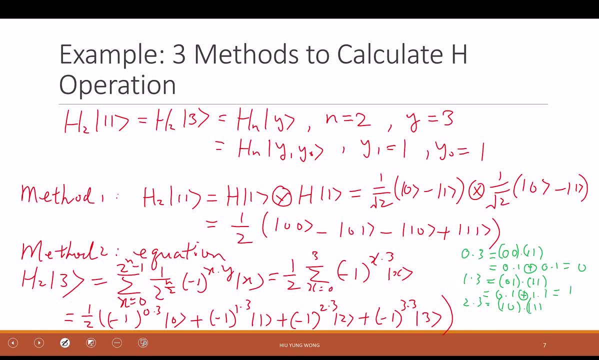 dot one one. so this is one dot one, exclusive zero dot one, and of course, this is one, and similarly, three dot three. you will find that is equal to zero. okay now, so if, if this is zero, then what is this term? zero dot three is zero. this is what? oh my god. 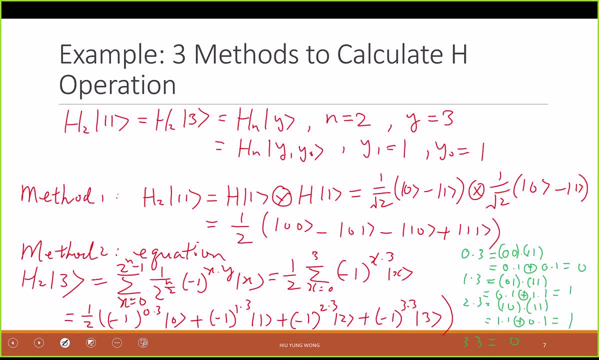 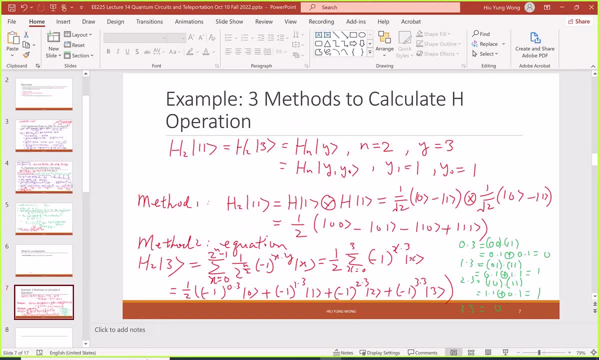 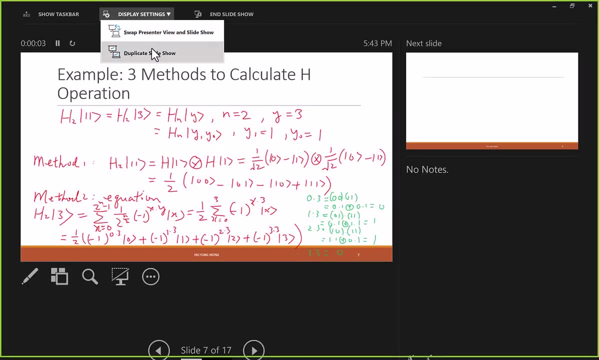 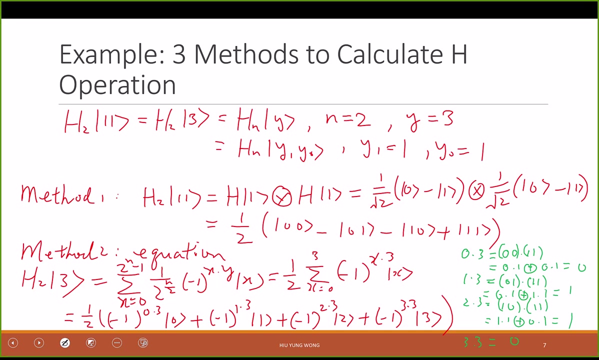 if the zero dot three is zero, what is negative? one to the zero, to the power zero, what it will be? plus one, right, am i right? so this become, oh, i see, plus one. how about the second term? negative one, negative one plus one right, so they are the same. 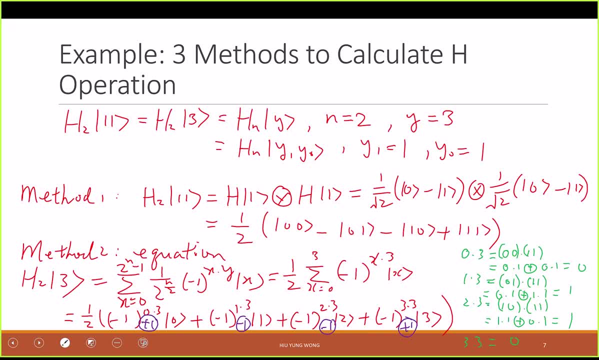 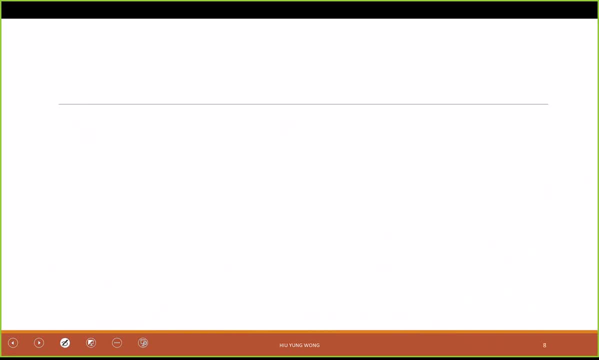 say: okay, right, so so do numerical substitution i will ask you to do in homework. that's how you understand better. okay, let me introduce the last method, but you know that already. just use matrix. right, you can use many things. the result has to be the same. okay, what is h2? 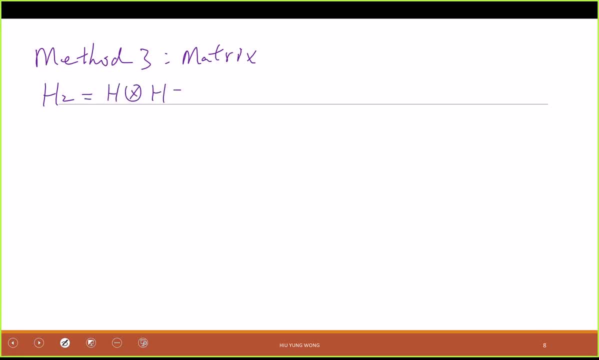 in matrix form is h tensor product h. what is h? square root? one, one, one negative one, try to memorize it. and the product one over square root two, one, one, one negative one. right, and how do you do it? well, this becomes one over two and you just copy one one, one negative one. 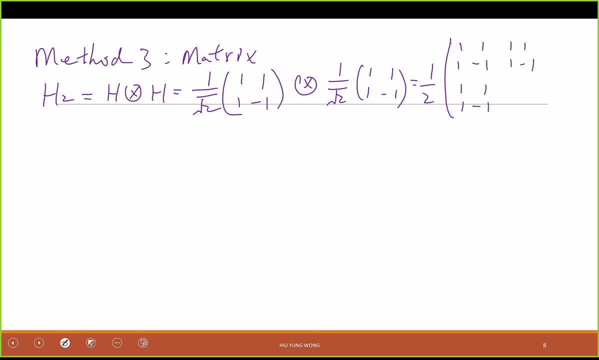 one, one, one, negative one. one, one, one negative one. and then the last one is negative one multiplied by a. so it's negative one, negative one, negative one one. do you see this? because i'm doing negative one times this whole thing. this becomes this block, right? remember tensor product? this one multiplies this whole thing. then you have this right.